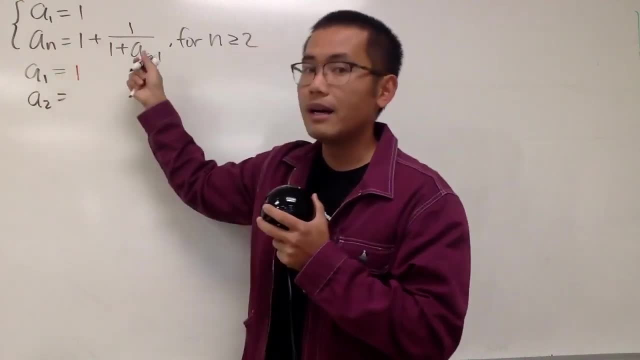 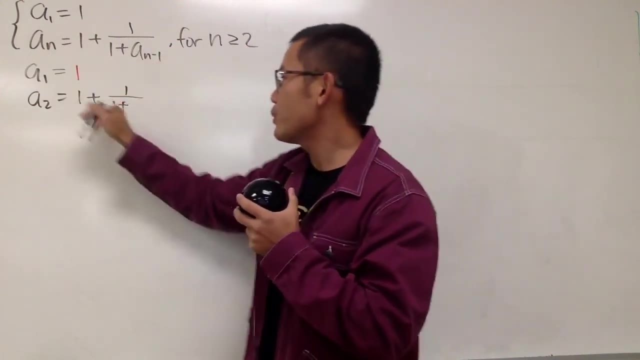 Now to get a2, we will have to utilize this formula, which says 1 plus 1 over 1 plus the previous term. So we have to look here, which is this: 1.. And now we can just add this up: this is 1 half plus 1, which is going to be 3 half, right here. 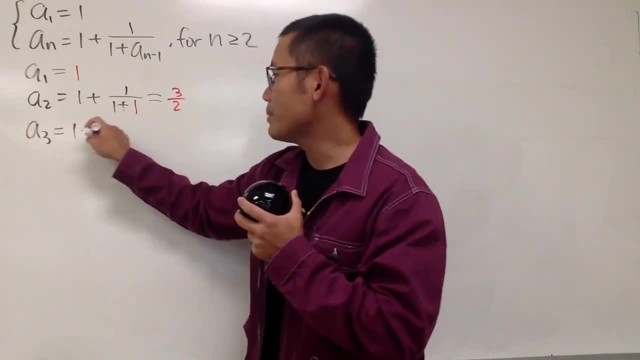 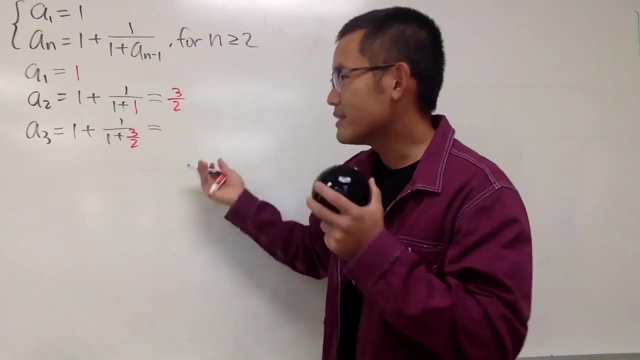 And, of course, keep on going This right here. a3, is going to be 1 plus 1 over 1 plus the previous term, which is 3 half- Just put it down here- and we are dealing with some complex fractions, but it's not so bad. 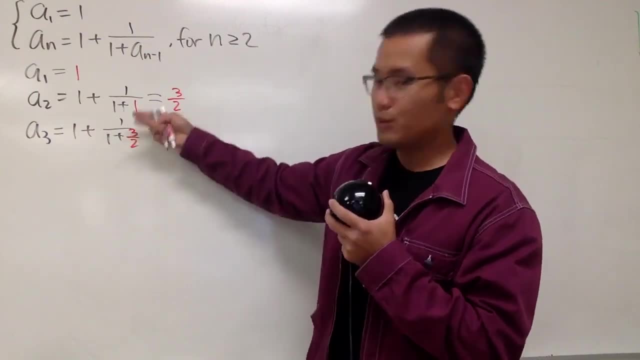 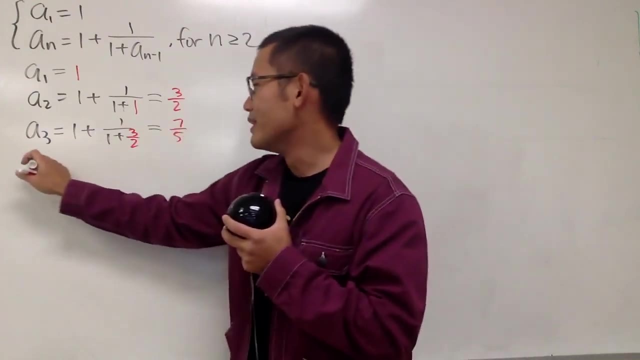 To do this. of course, this is going to be 5 half. do the reciprocal. it's 2 over 5, plus 1, it's going to be 7 over 5,. like this right, And let's do one more. 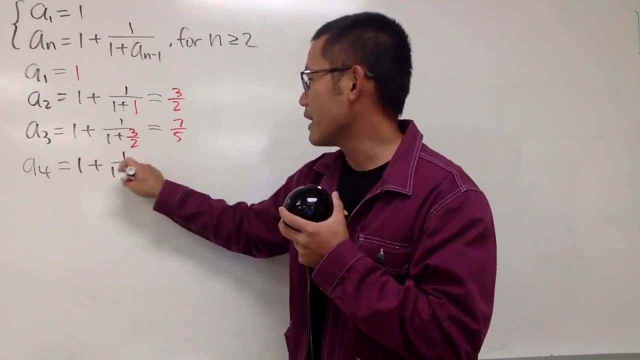 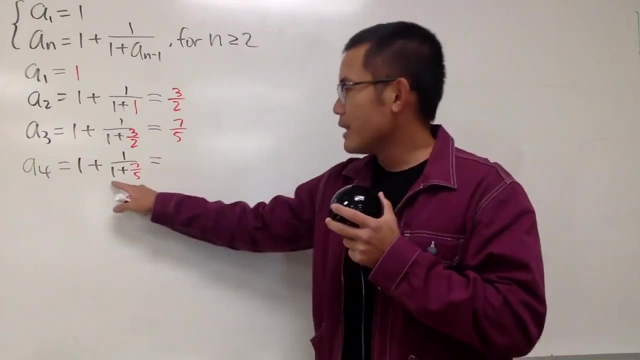 a4 is equal to 1 plus 1 over 1, plus 7 over 5,. right here, And let's see if we can do this in our head or not. Okay, plus 1, it's going to be 12 over 5, do the reciprocal: it's going to be 5 over 12,. 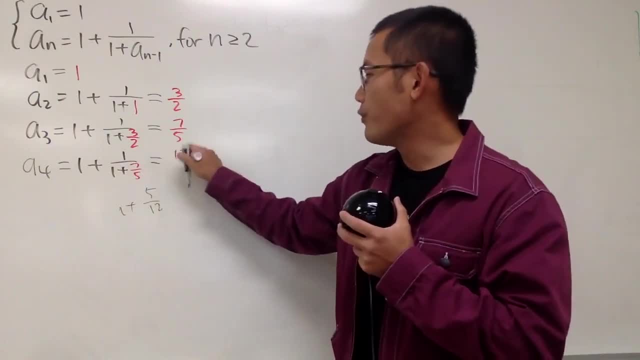 and then we add 1 to that, it's going to be 17 over 5.. And then we add 1 to that, it's going to be 7 over 12, like this right. So that's the idea. 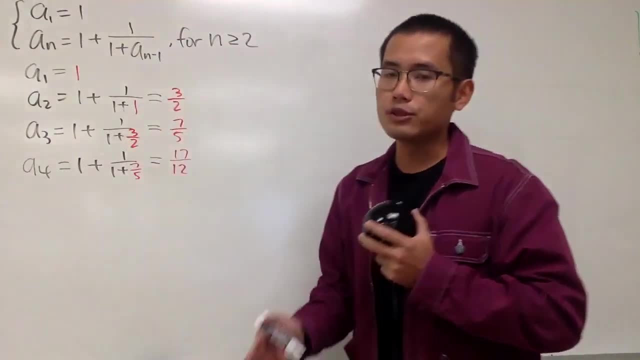 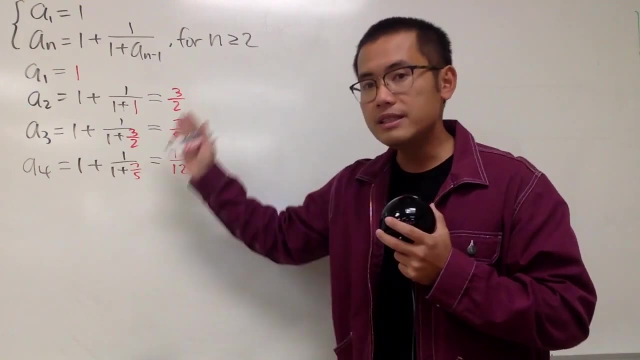 First thing. first, as you can see, all these numbers right here are just going to be fractions and, more specifically, they are rational numbers, because we have a whole number over a whole number. These numbers are rational And let's see, I don't want to deal with fractions anymore. 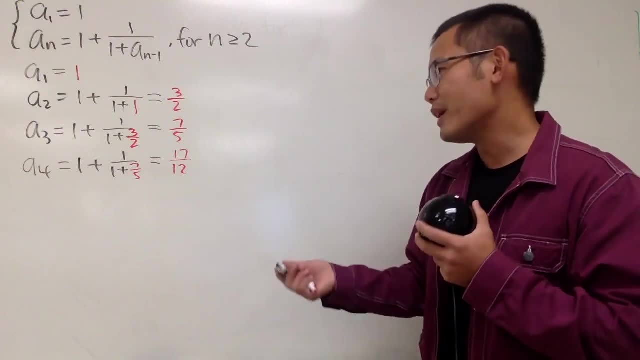 and also I want to see how big the numbers are in an easier way. so I will just tell you guys the decimal versions right here. So I will just tell you guys the decimal versions right here: 1 is 1, of course. 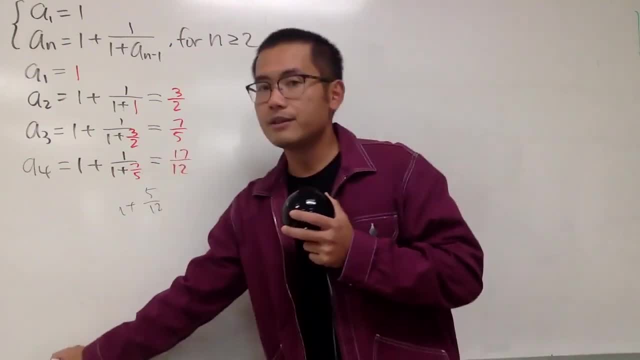 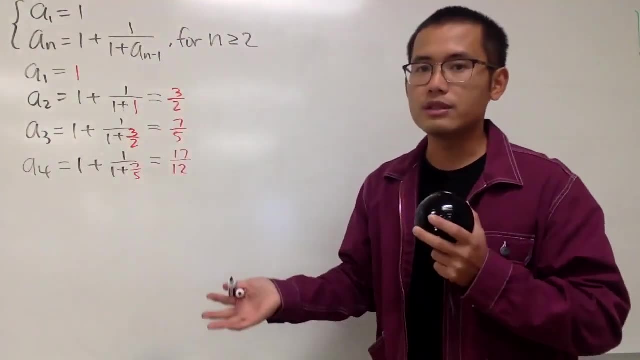 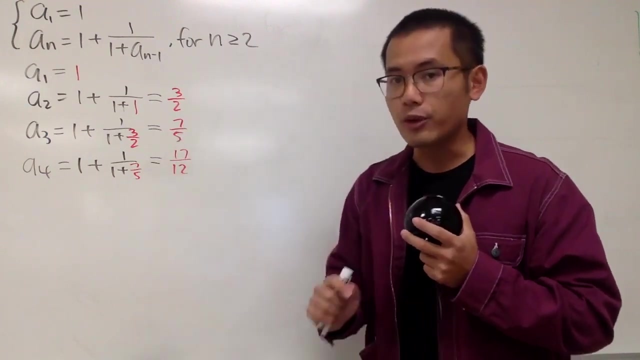 over 12, like this, right? so that's the idea, first thing. first, as you can see, all these numbers right here are just going to be fractions and, more specifically, they are rational numbers, because we have a whole number over a whole number. these numbers are rational and let's see, um, i don't want. 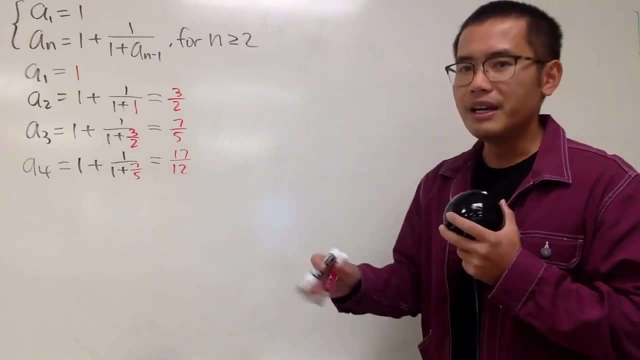 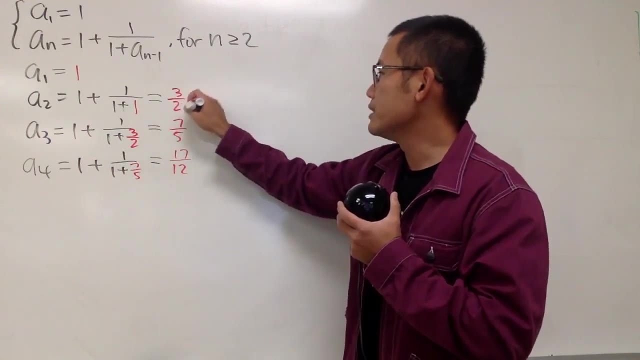 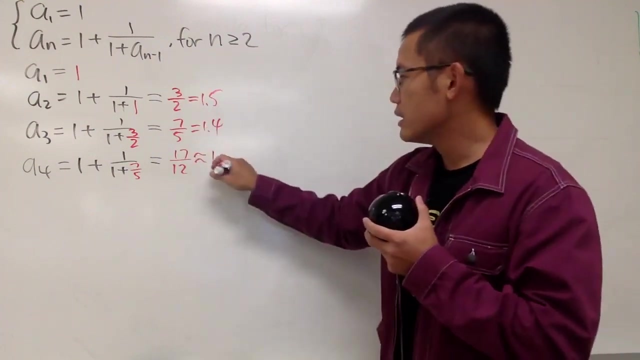 to deal with fractions anymore and also i want to see how big the numbers are in a easier way. so i will just tell you guys the decimal versions right here. one is one, of course: this right here is equal to 1.5, this right here is equal to 1.4 and this right here is approximately equal to 1.41. and 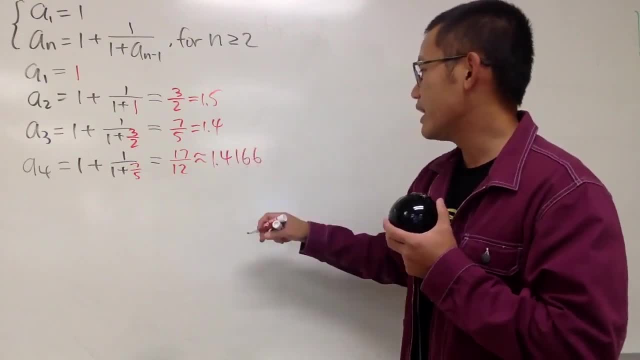 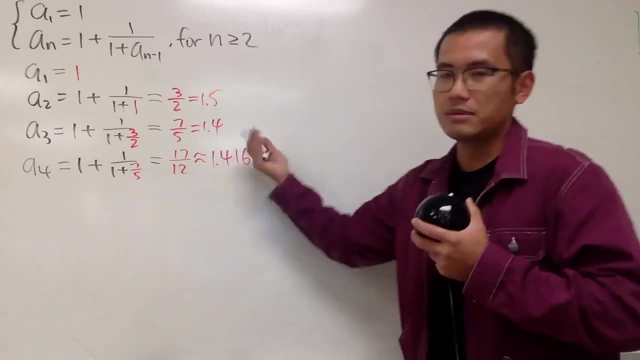 let me just use a couple more digits. let's say six, six, and i'm just going to cut it off, i'm not going to run, okay, so just six, six and one more, right, and then just dot, dot, dot, because it keeps on going forever. all right, so now you see, we go from one and you go up. 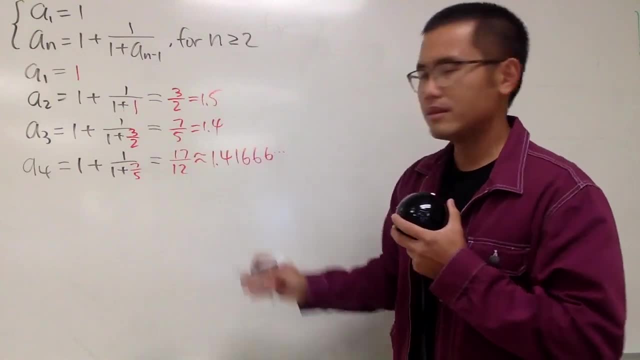 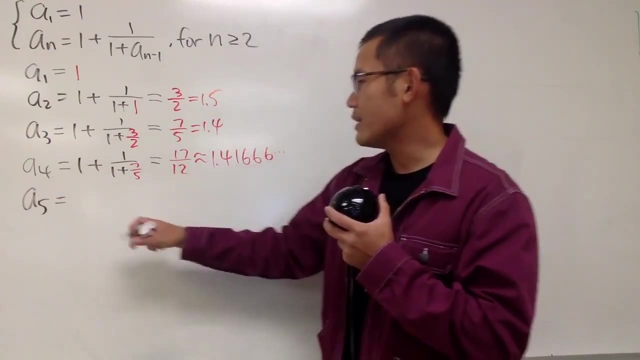 huh, it goes up and then it went down and then it goes up. it's kind of weird. huh, let's do one more. let's see what happens if we have a5. of course, this is going to be that, and i'll just put this down right here for you guys. i'll just put this down as 1 plus 1 over 1 plus, which is a 17 over 12.. 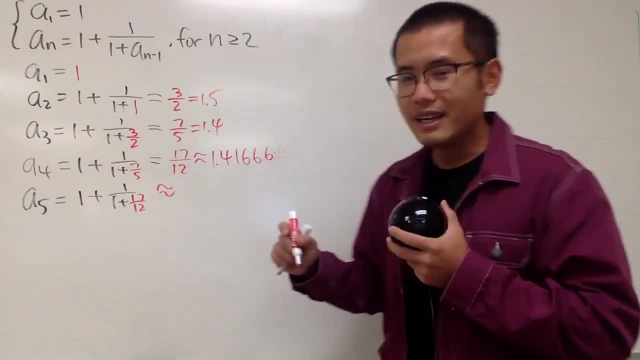 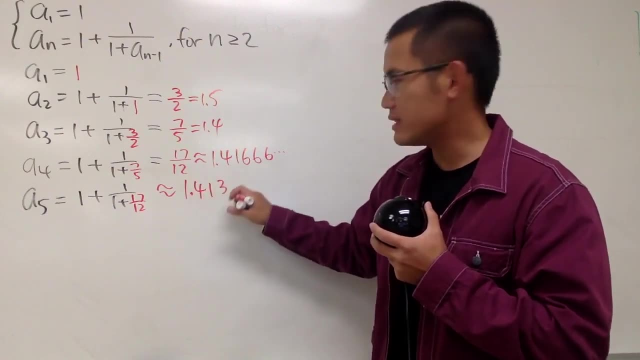 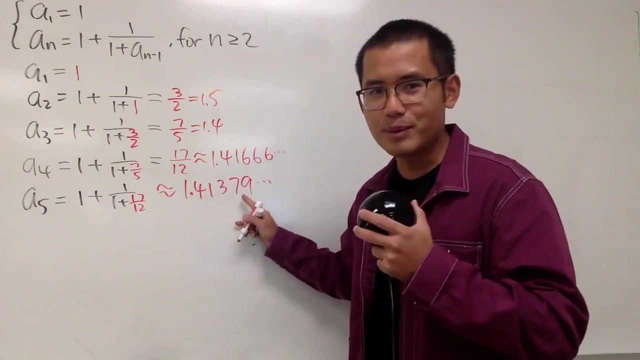 but this time i'll just tell you guys the decimal for this. it's going to be what this is going to be: 1.4137, 9 and then ta, ta. so let me just check. yes, i have the answers on the screen because i can. 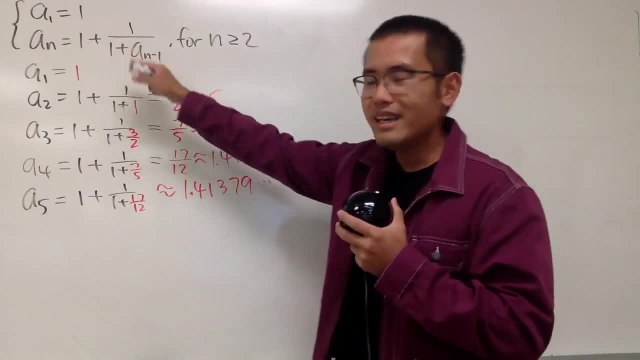 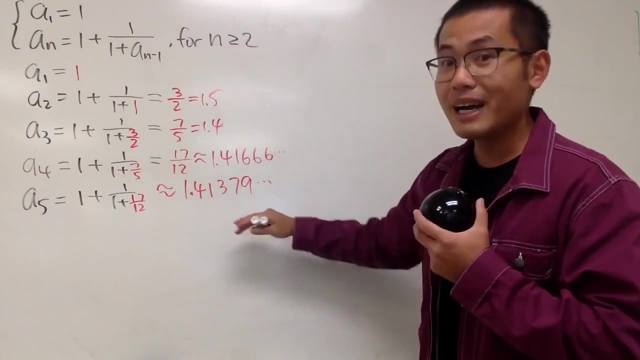 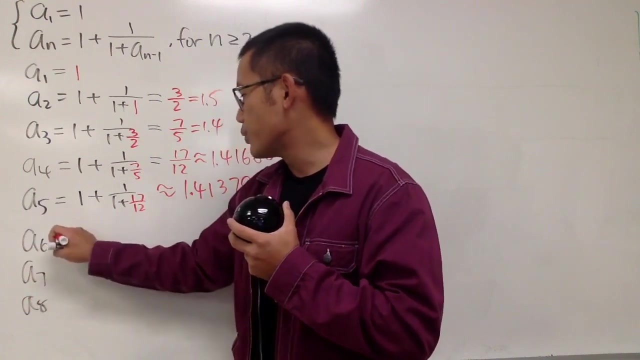 memorize all these digits, okay, so you see one and then goes up, and then one down, and then, well, it goes down and then goes up and then goes down. ah, interesting. and now i'll just tell you guys the rest of the answers, that's the A6, A7 and A8. so you pretty much do the following. 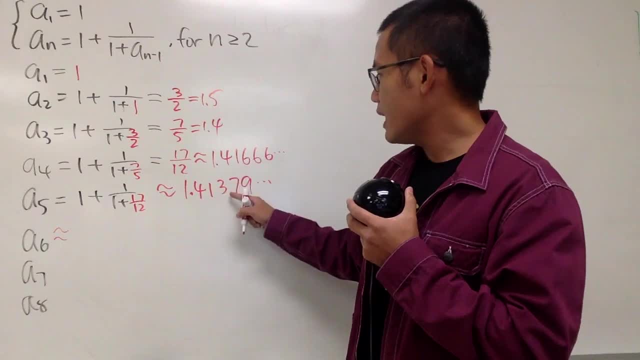 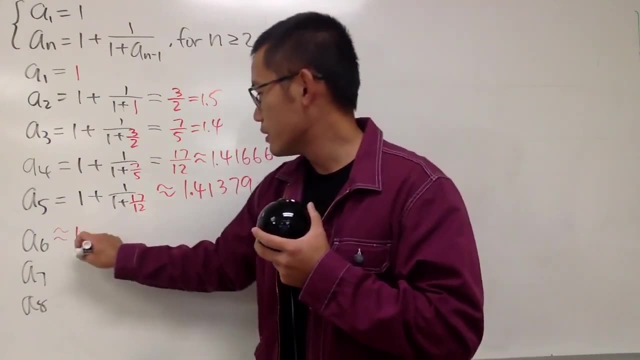 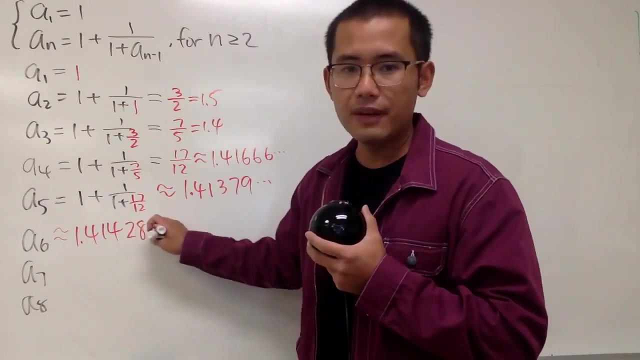 so, A6, you can guess it. we went down earlier, so it's going to go up and then up, you guys get the answers, And that's in fact the pattern, and it's going to be 1.414.. Huh, interesting: 1.414, 2, 8, 5, and so on, so on, so on. 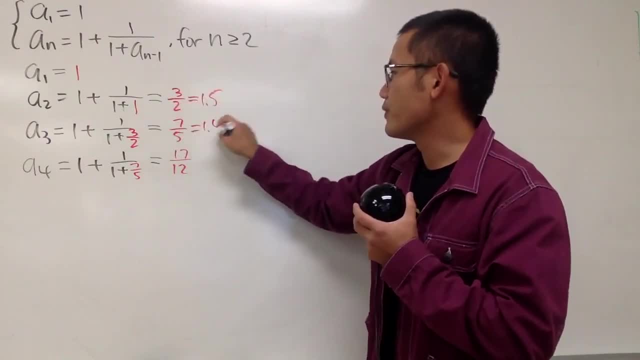 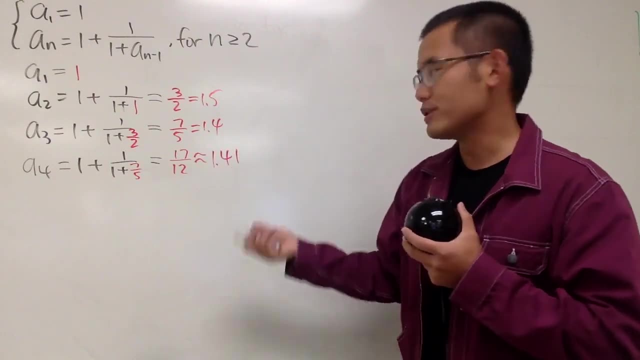 This right here is equal to 1.5,, this right here is equal to 1.4, and this right here is approximately equal to 1.41,. and let me just use a couple more digits. let's say 6,, 6,. 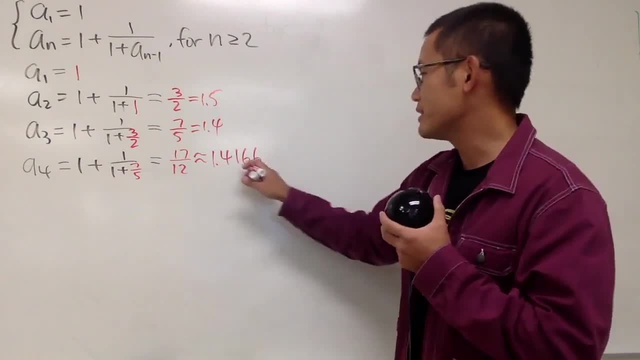 and I'm just going to cut it off. I'm not going to do it wrong, okay, So it's just 6,, 6, and one more, right, And then just dot, dot, dot, because it keeps on going forever. 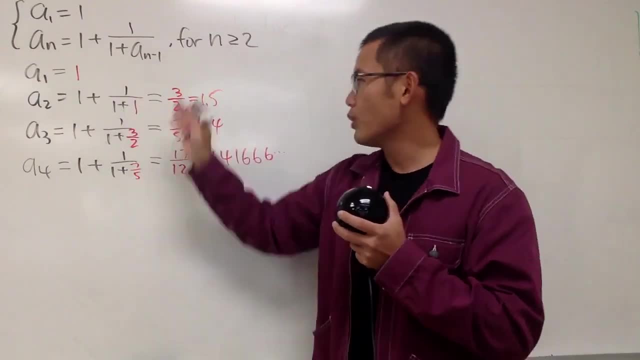 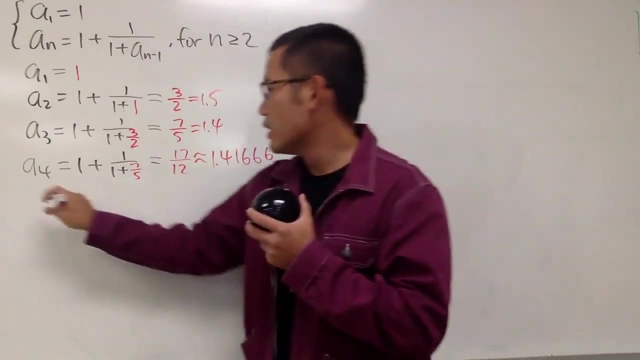 All right. so now you see, we go from 1, and it goes up. huh, It goes up. and then it went down, It goes up. it's kind of weird. huh, Let's do one more. let's see what happens. 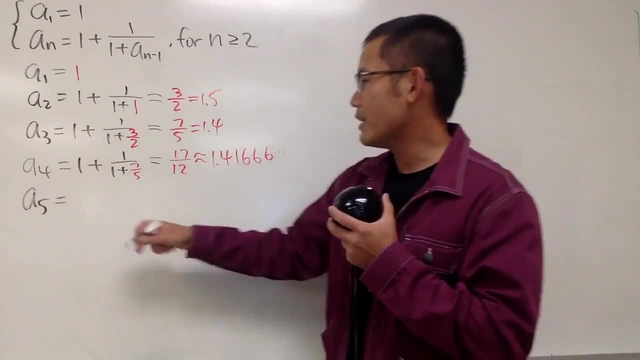 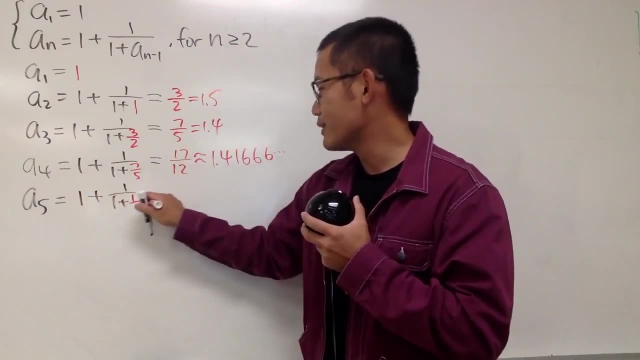 If we have a5, of course this is going to be that and I'll just put this down right here for you guys. I'll just put this down as 1 plus 1 over 1 plus, which is a 17 over 12,. 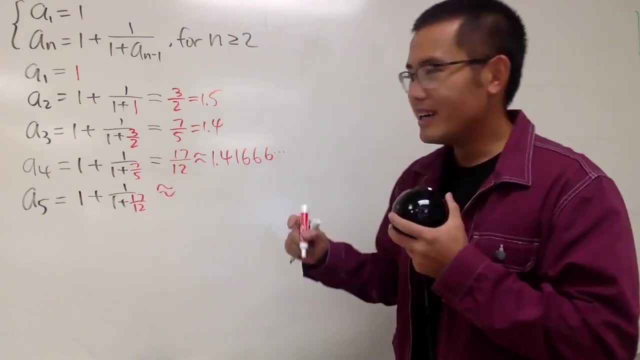 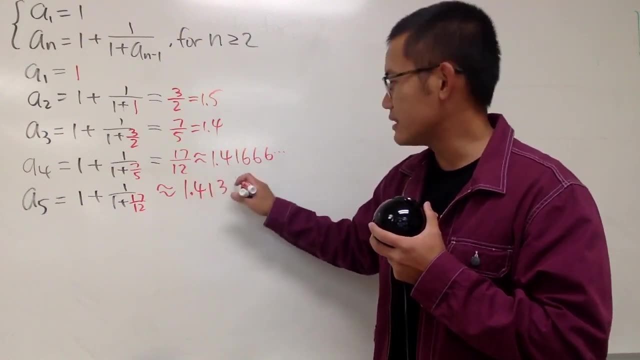 but this time I'll just tell you guys the decimal for this. It's going to be what. This is going to be 1.41379,. and then dot dot dot. So let me just check. Yes, I have the answers on the screen. 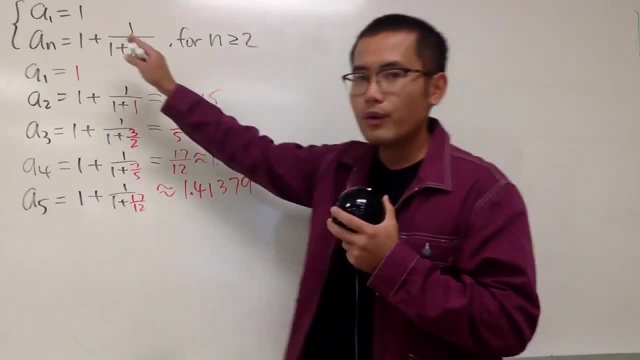 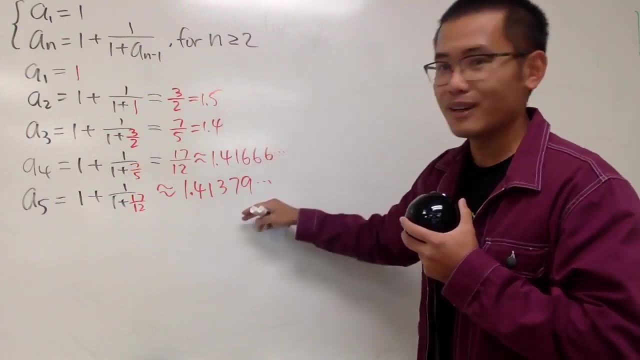 because I can memorize all these digits. Okay, so you see 1, and then goes up, and then went down, and then goes down, and then goes up and then goes down. Huh, interesting, And I'll just tell you guys the rest of the answers. 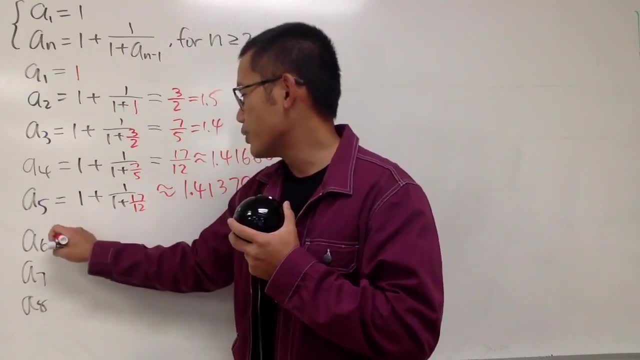 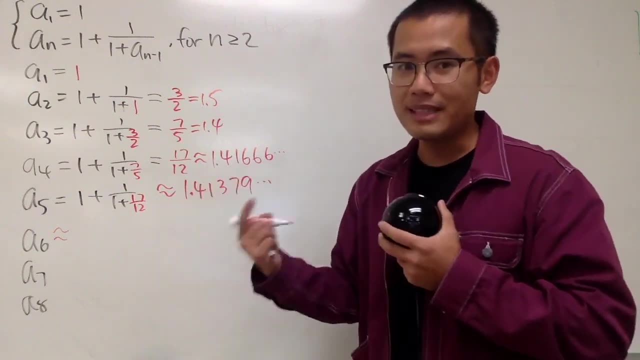 that's the a6, a7, and a8.. So you pretty much do the following. So a6, you can guess it. It went down earlier, so it's going to go up, and that's in fact the pattern. So, a6,, you can guess it, We went down earlier, so it's going to go up, and that's, in fact, the pattern. So, a6,, you can guess it, We went down earlier, so it's going to go up, and that's, in fact, the pattern. 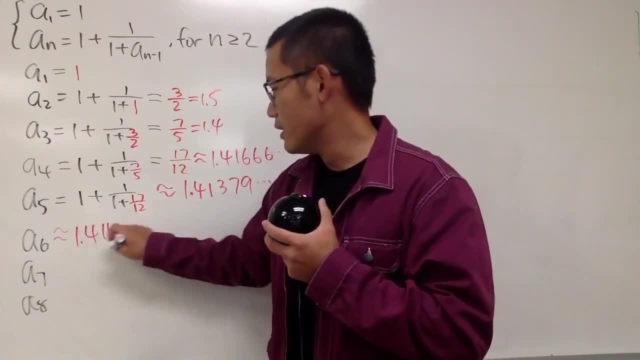 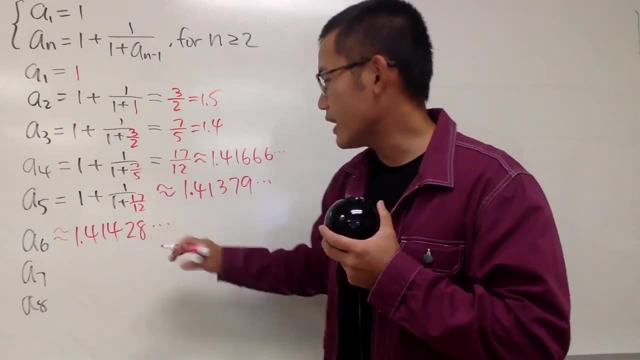 So a6, you can guess it. We went down earlier, so it's going to go up, and that's in fact the pattern. It's going to be 1.414.. Interesting 1.414285, and so on, so on. 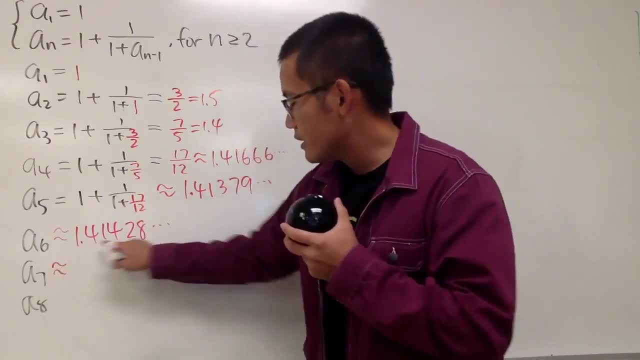 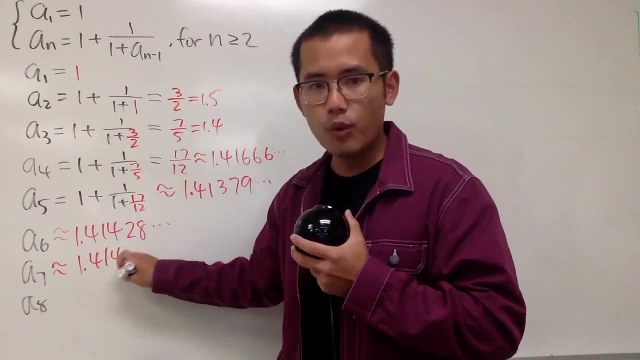 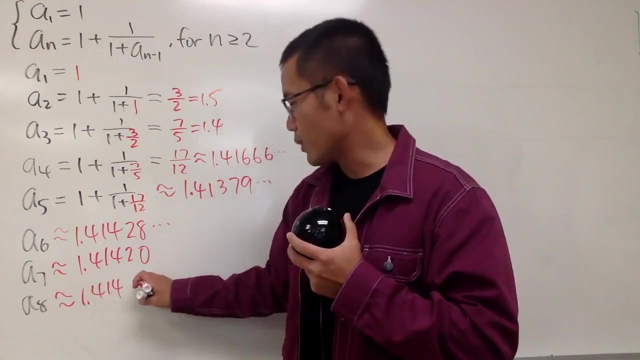 Again, I'm not wrong there. I'm just writing down the first five digits after the decimal point Right here. so that's 1 point and five digits, And then next we have 1.41420.. And here a8 is 1.41421. 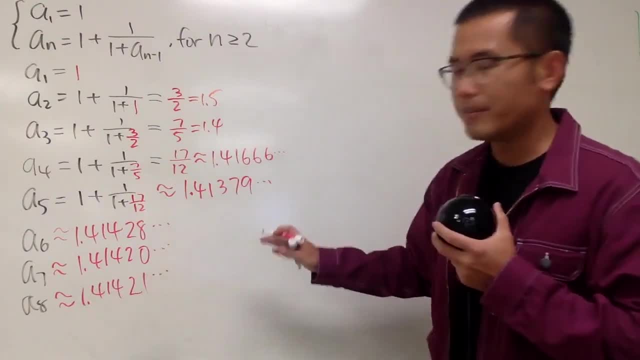 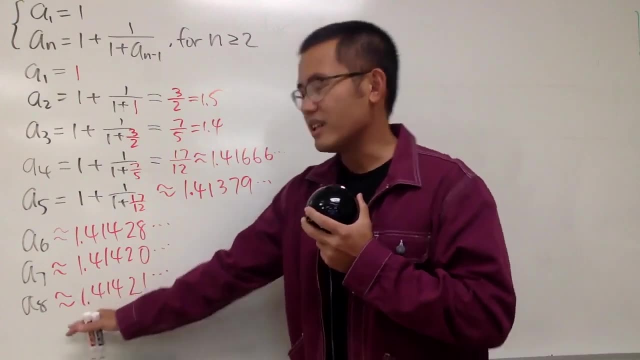 Huh, As you can see, it looks like this number is actually converging to about 1.414, because you see that I don't think the next one is going to be that big of a difference, isn't it? So very nice, and here is the deal. 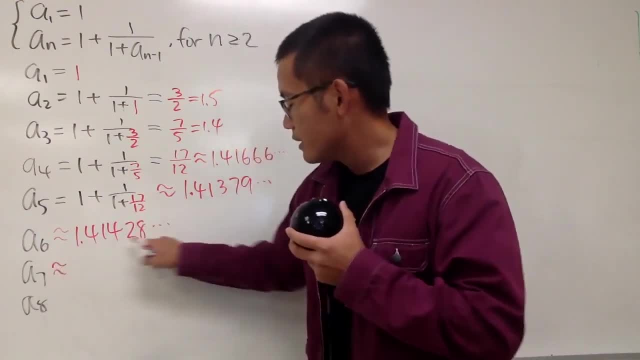 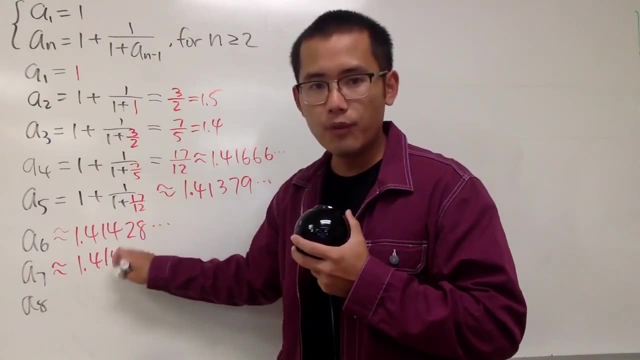 Again, I'm not wrong there. I'm just writing down the first five digits after the decimal point right here. So it's 1.5 digits, And then next we have 1.41420, and here AA is 1.414. 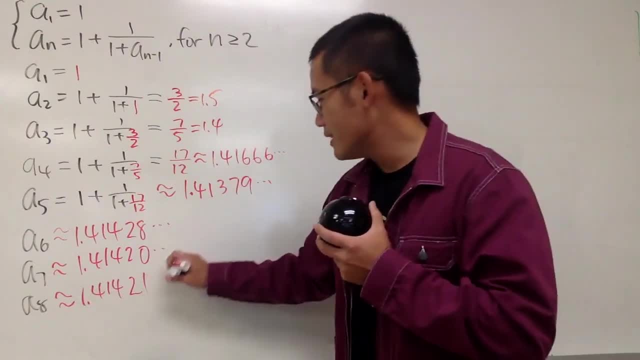 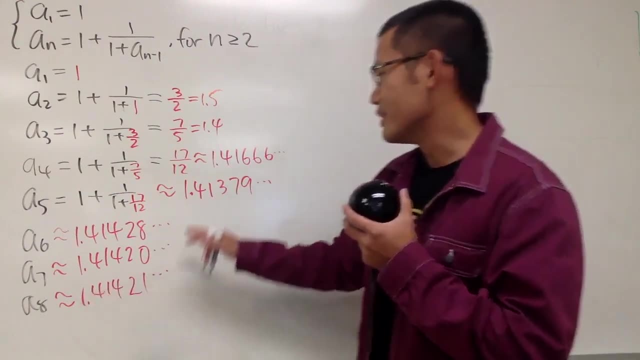 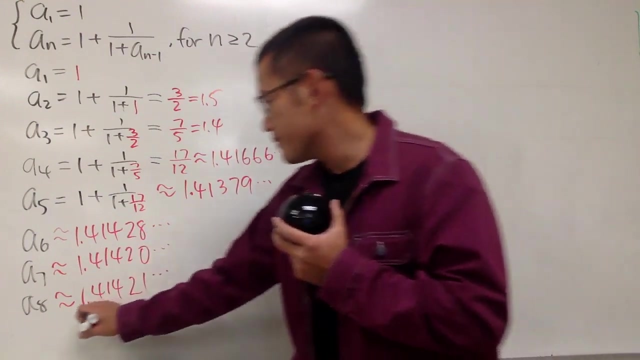 Ah, as you can see, it looks like this number is actually converging to about 1.414, because you see that I don't think the next one is going to be that big of a difference, isn't it? So very nice, and here is the deal. this is the list of the first eight terms. 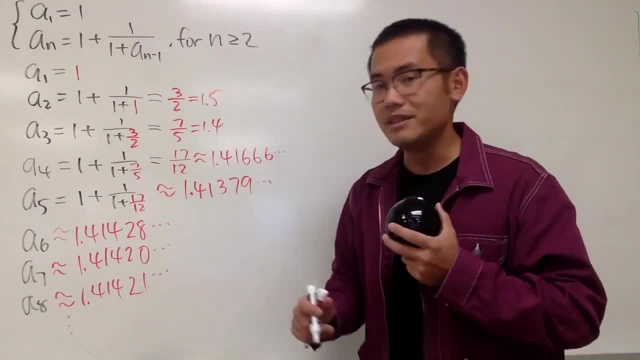 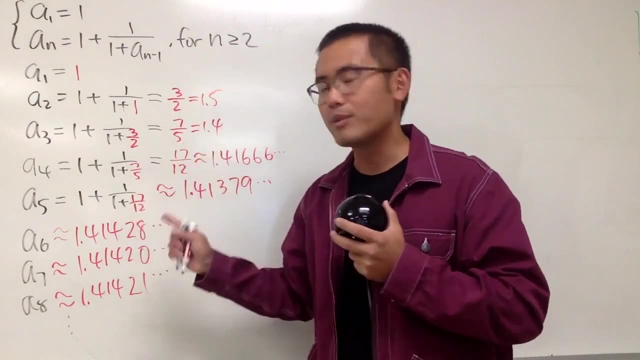 And we're going to find out like what this is going to converge. to Keep in mind, though, every single You can see here there were fractions, again rational numbers, but this number doesn't look rational at all. 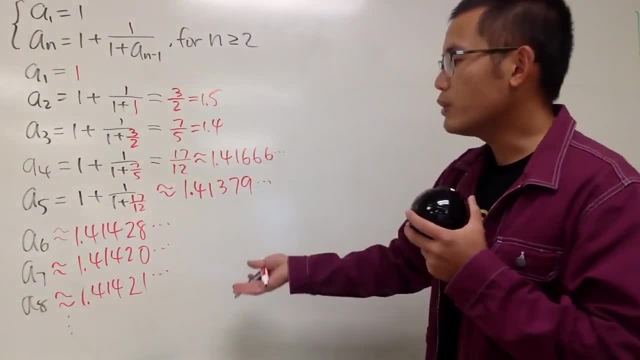 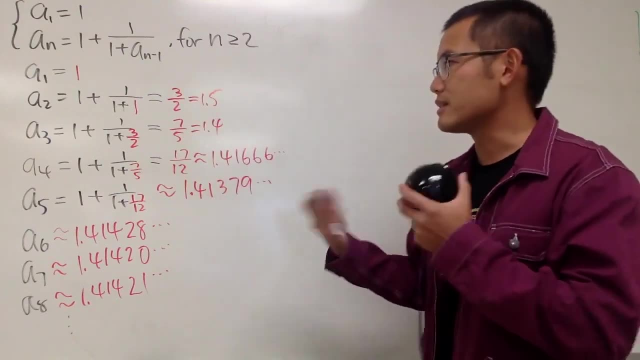 So here is the deal. In fact, to show that this actually converges, you have to do more like technical work, such as you have to prove that this is increasing, decreasing, etc. or bounding above whatsoever. but, like you know, I'm not going to worry about that too much because this is just an introductory question. 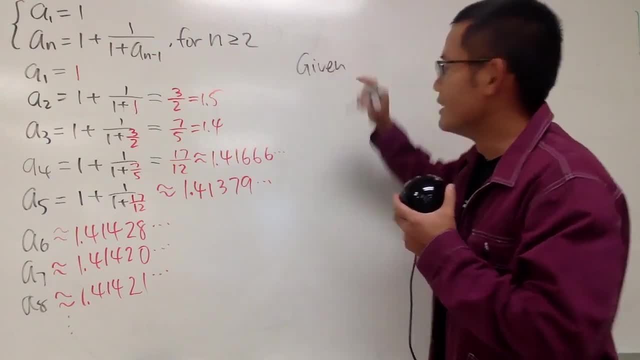 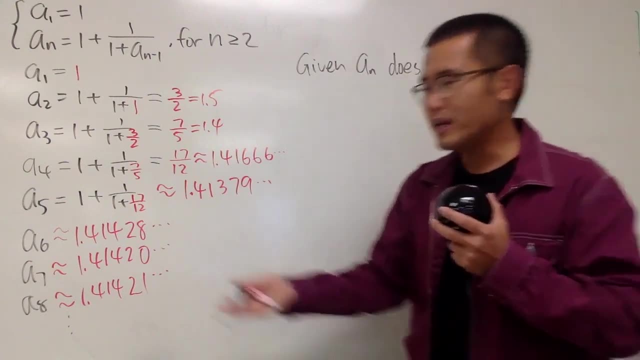 I will tell you guys that, given which I actually gave you guys this scenario, given AN does converge, So you know, in the end you actually end up with a finite result. all right, Now we are going to find out what the limit of AN is. 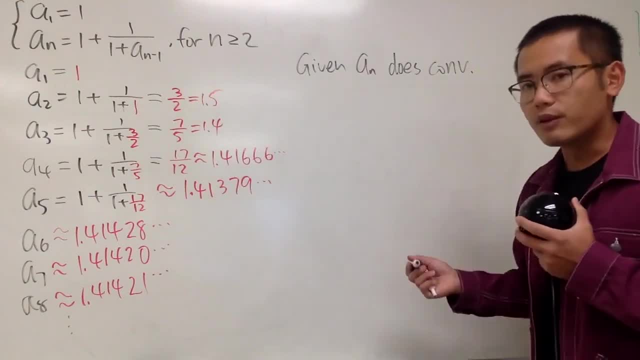 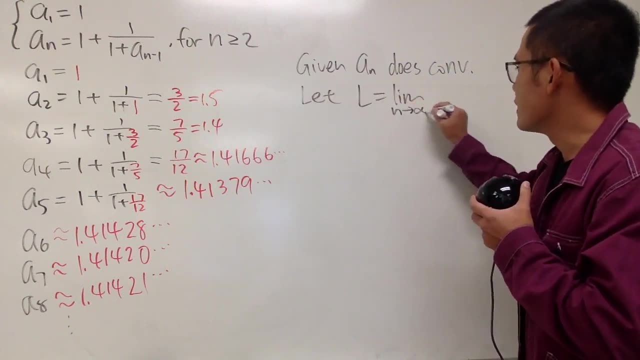 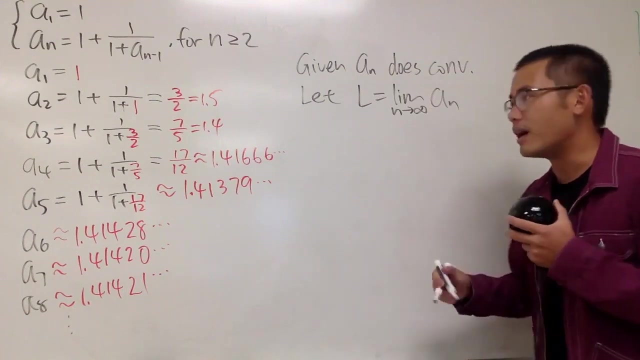 This is how, Given this right here, does converge. So I would just say: let L equal to the limit, as N goes to infinity of AN, because of course AN does converge. And now here is perhaps the slightly tricky part. 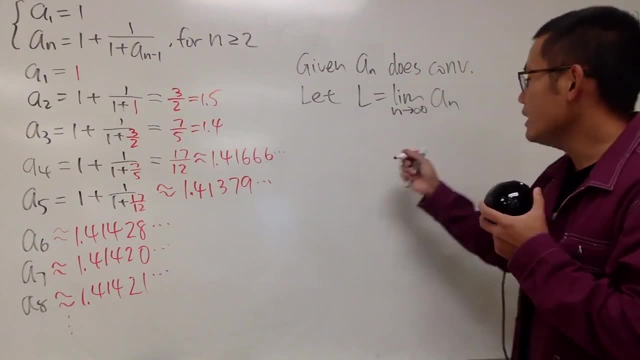 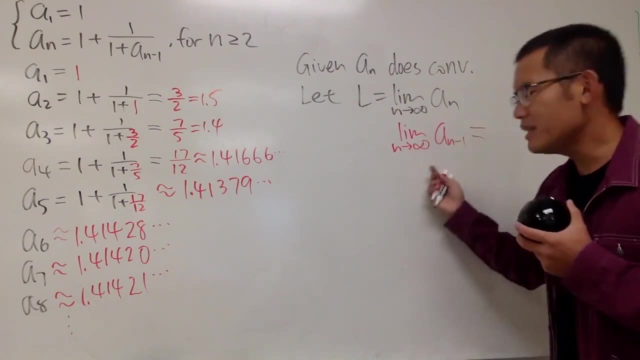 If AN converges, converges to L. well, what if we take the limit, as N goes to infinity, of AN minus 1?? If you look at this, this is not just off by 1, but the idea is that, well, if AN goes to L, 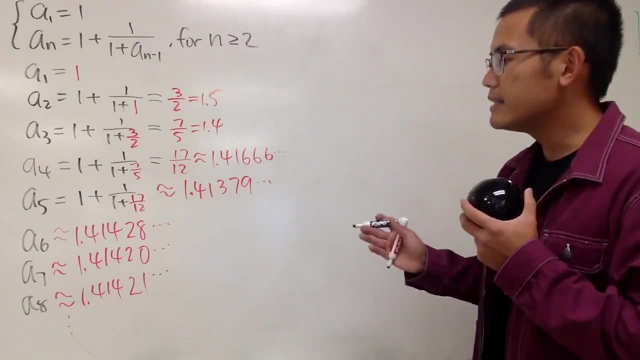 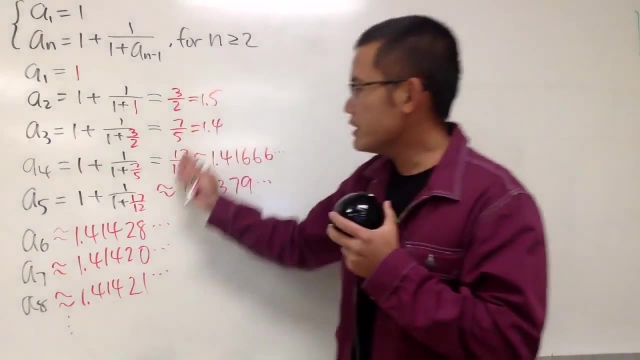 This is the list of the first eight terms, And we're going to find out what this is going to converge. to Keep in mind, though, everything here they were fractions, again rational numbers, but this number doesn't look rational at all. 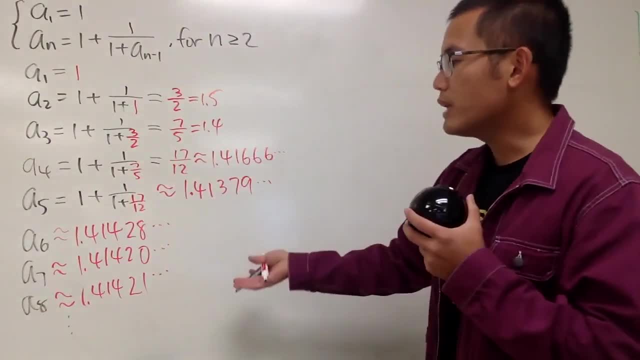 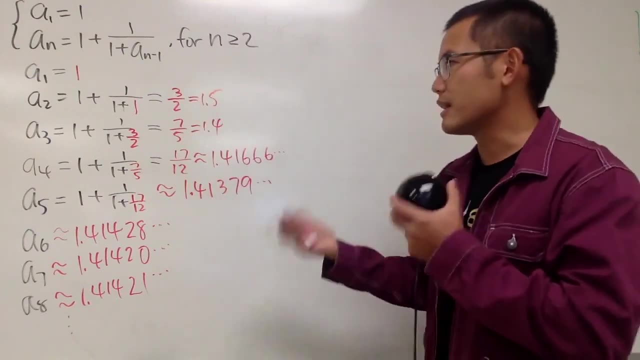 So here is the deal. In fact, to show that this actually converges, you have to do more, like a technical work, such as you have to prove that this is increasing, decreasing, etc. or bounding above whatsoever. but, like you know, I'm not going to worry about that too much because this is just an introductory question. 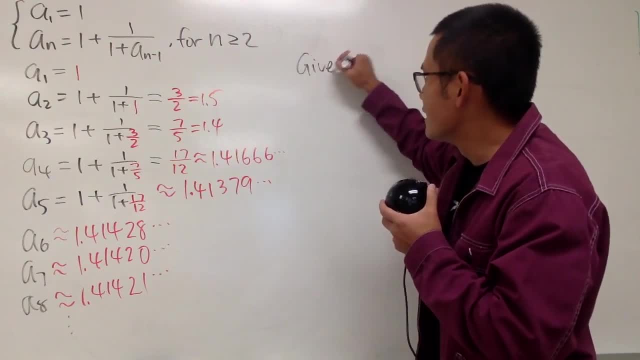 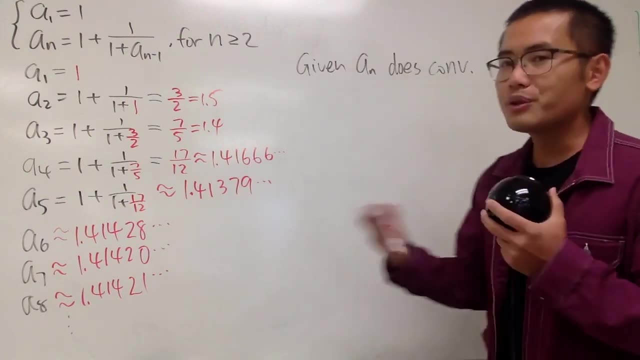 And I will tell you guys that, given which I actually gave you guys this scenario, given a n does converge, so you know, in the end you actually end up with a finite result. alright, Now we are going to find out what the limit of a n is. 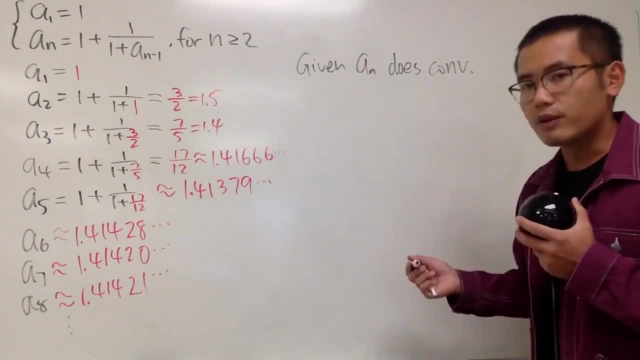 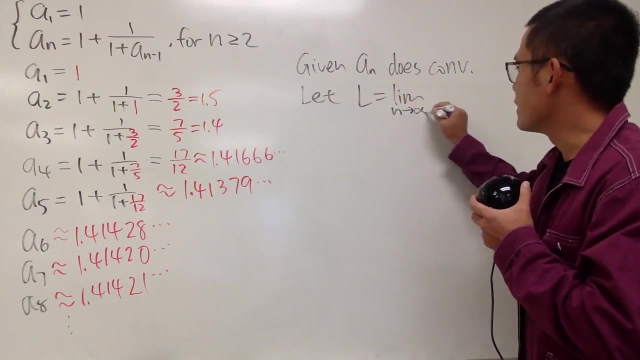 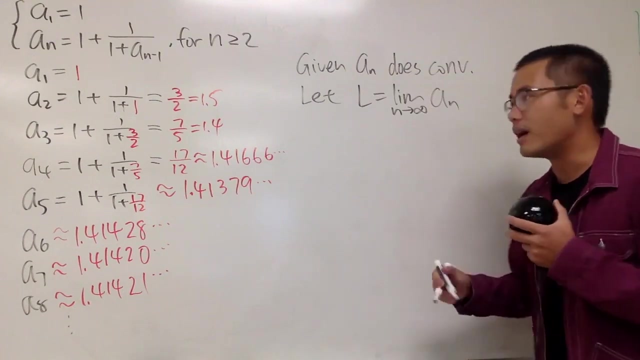 This is how, Given this right here, does converge. so I will just say: let l equal to the limit, as n goes to infinity, of a n, because of course a n does converge. And now here is perhaps a slightly tricky part. 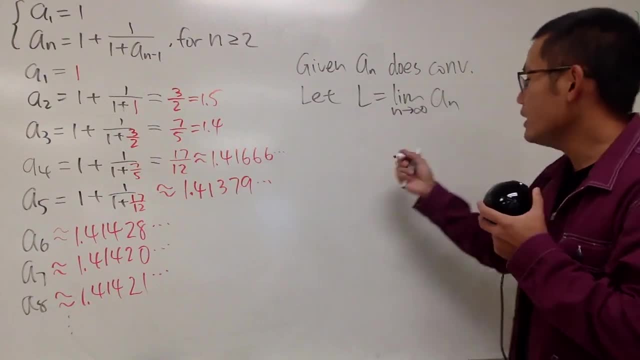 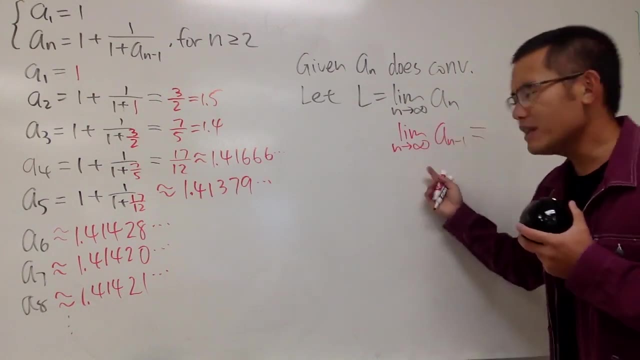 If a n converges to l? well, what if we take the limit, as n goes to infinity, of a n minus 1?? If you look at this, this is not just off by 1, but the idea is that. well, 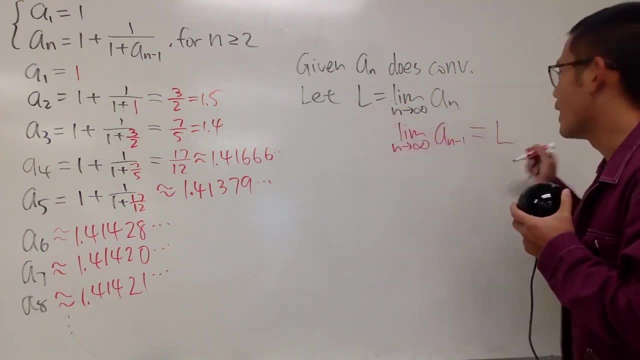 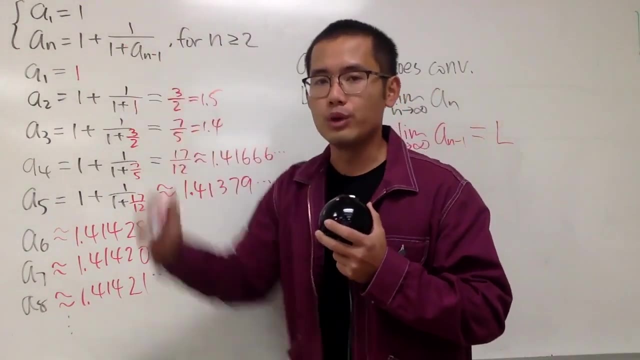 if a n goes to l, a n minus 1 will go to l as well. That's the idea, And the reason I bring this up is because we actually have to look back to our recursive formula, and from there I will just write this down again. 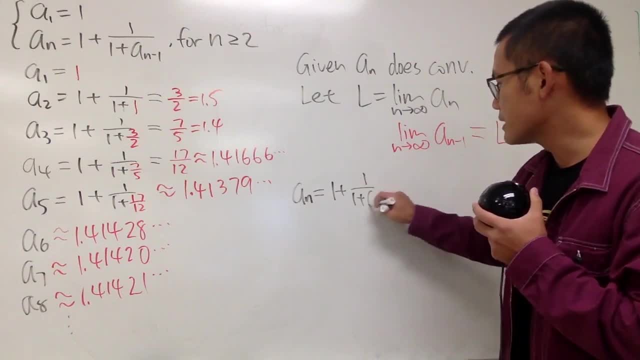 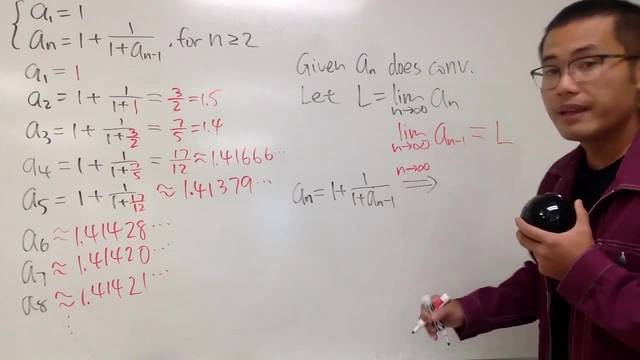 a n equals 1 plus 1 over 1 plus a n minus 1.. Well, we can just take the limit as n goes to infinity and the idea is that this right here will go to l, because right here we said so. 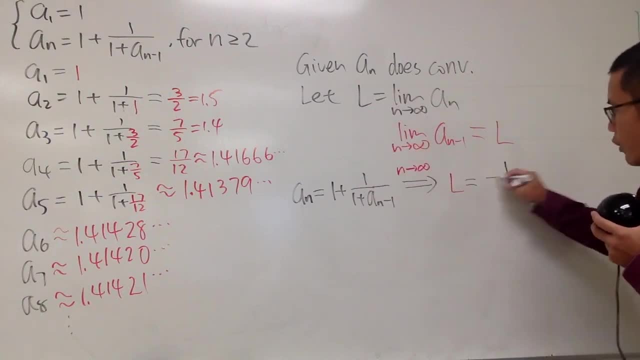 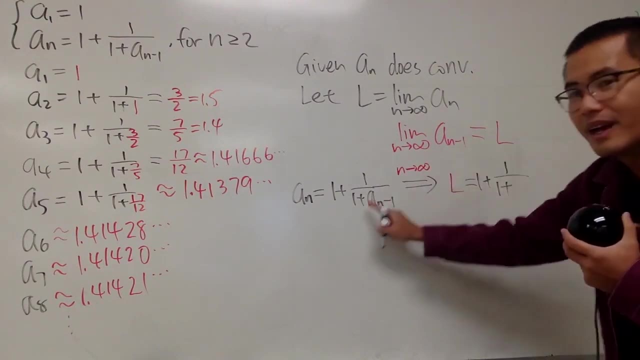 And then, of course, the rest we get. this is equal to: and we have 1 over, well, actually 1 plus 1 over. there are so many 1s, and then 1 plus this thing, a n minus 1, which I wrote it down and l like this: 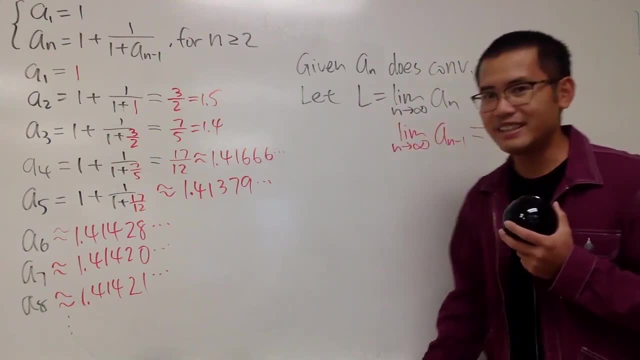 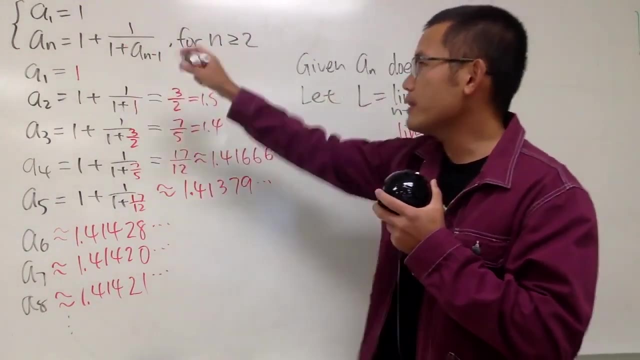 AN minus 1 will go to L as well. That's the idea, And the reason I bring this up is because we actually have to look back to our recursive formula and from there I will just write this down again Again: AN equals 1 plus 1.. 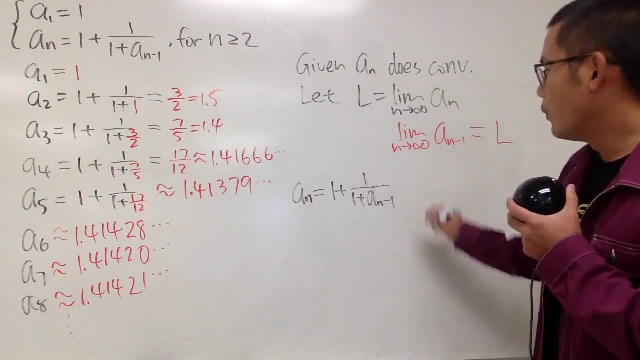 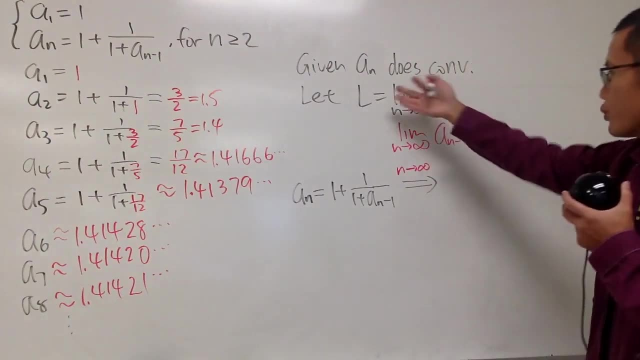 AN equals 1 over 1 plus AN minus 1.. Well, we can just take the limit as N goes to infinity And the idea is that this right here will go to L, because right here we said so, And then of course the rest we get. this is equal to and we have 1 over. 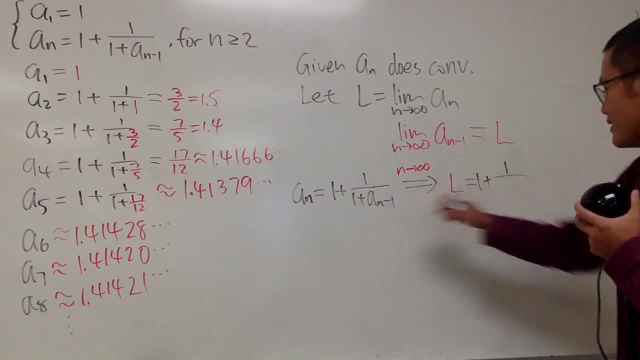 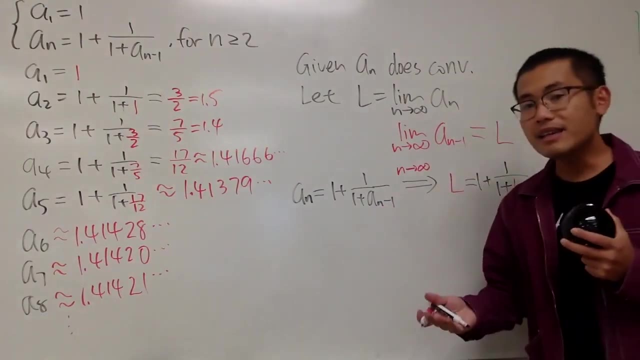 well, actually 1 plus 1, over there are so many 1s, And then 1 plus this thing, AN minus 1, which I wrote it down and L like this: This kind of technique will work If we end up. 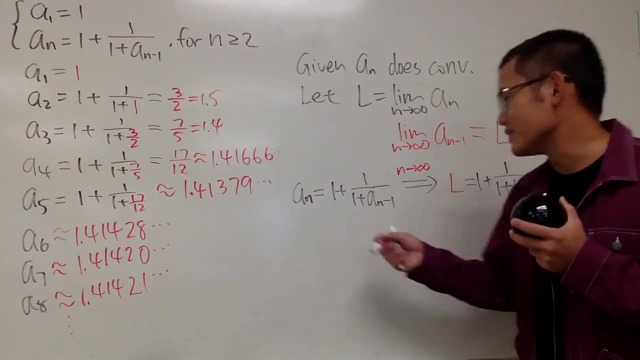 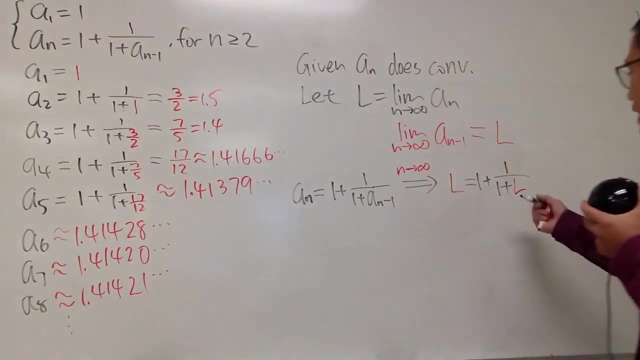 Well, it's a finite answer right here and then if it doesn't end up with any kind of weird situations. So of course, let's just figure this out. And to work this out, of course we can just multiply everybody by the lowest common denominator. 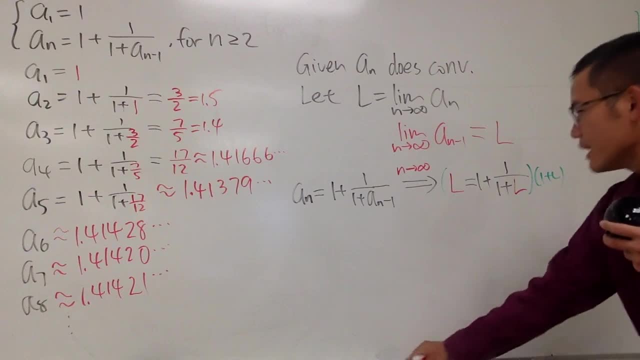 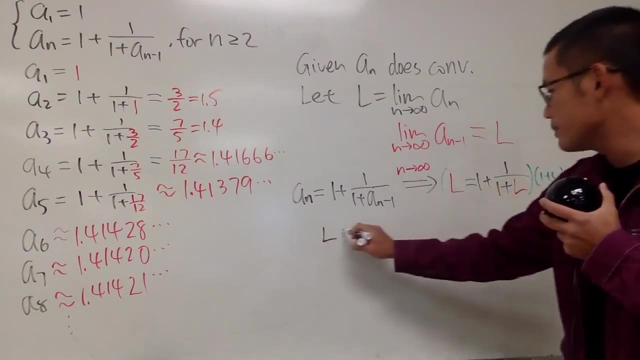 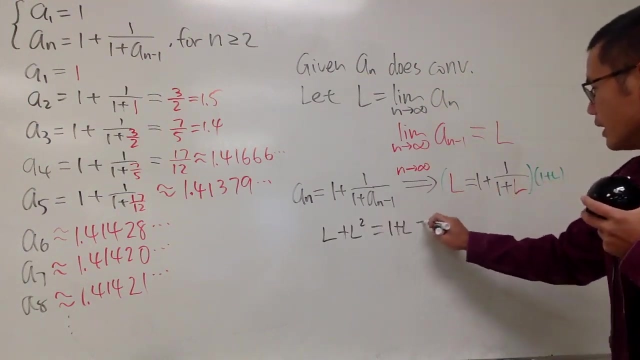 just the usual way. so 1 plus L, and we see that- Let me just put it down right here. We get this times that, which is going to be L times 1 plus L, squared, and that's equal to this times 1, which is 1 plus L. 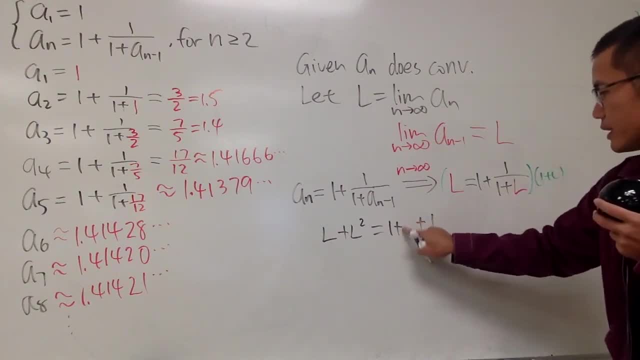 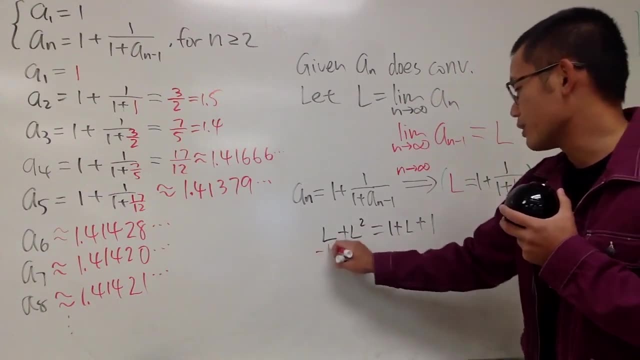 and we add this times that they cancel, so we add 1 to it. So again, I'm just multiplying things out. And now you see, we have the L on both sides, so we can minus L on both sides. 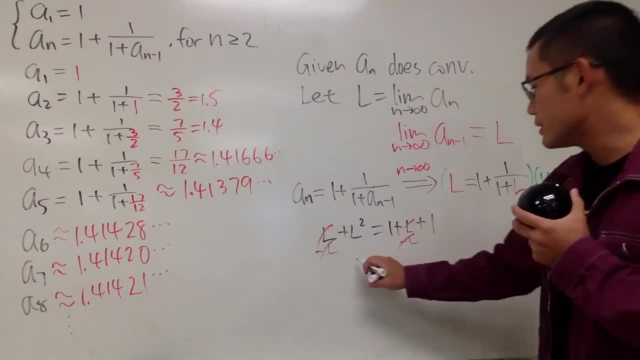 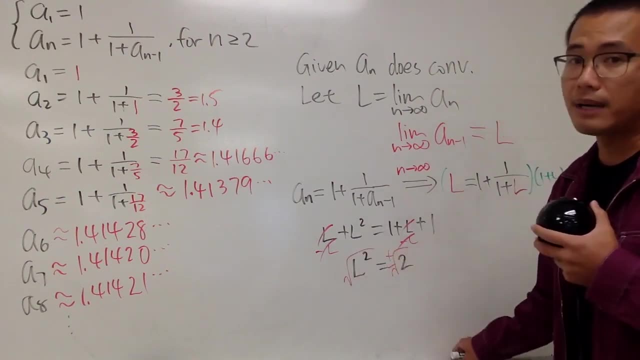 and that cancels out very nicely, right, And we end up with L squared. it's equal to 1 plus 1, which is 2.. And of course we can take the square roots on both sides. Usually you put on plus, minus. but if you look at all these numbers right here, 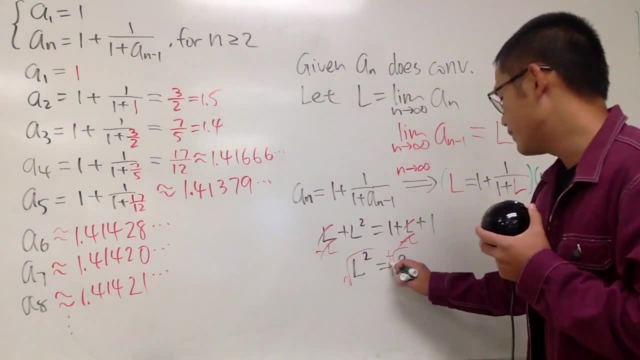 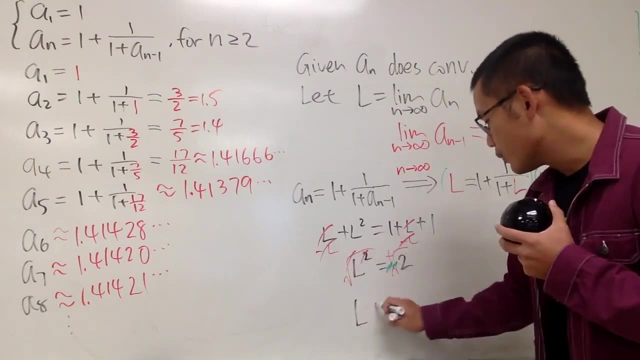 everybody's positive, there's no way to be negative. So in fact the negative doesn't matter. So in the end we are saying: this is a cancel of course L, which is the limit, as n goes to infinity, of a n.